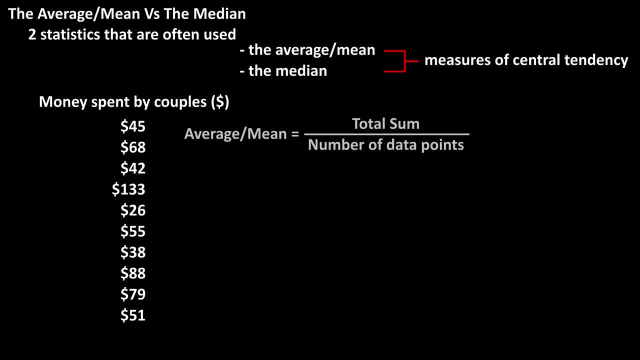 spent by 10 different couples at a restaurant. To calculate the mean or average, we add up all of the values and divide by the total number of values. Adding them up, we get 625 dollars and there are 10 total values. So 625 dollars divided by 10 equals 62 dollars and 50 cents. 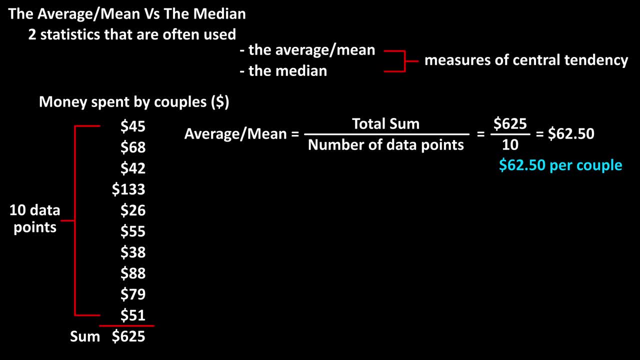 which is the mean or average spent per couple. Now for the median, which is the middle value, or between the middle values. Since we have 10 total values and even number of values, it will be between the middle values. We will arrange the values in ascending or increasing. 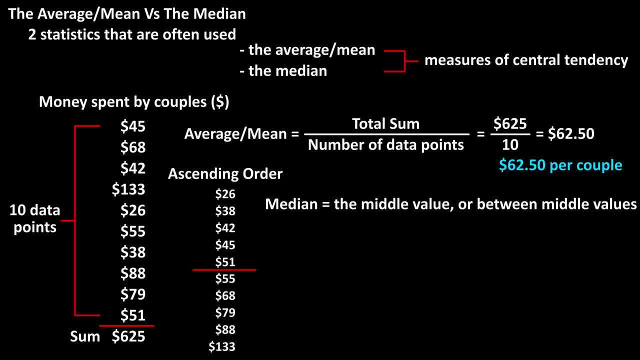 order. Draw a line here in the middle where we have five values lower and five values higher and add these two middle values together and divide that total by two, which gives us 53 dollars, which is our median. So we have an average of 62 dollars and 50 cents and a median of 53. 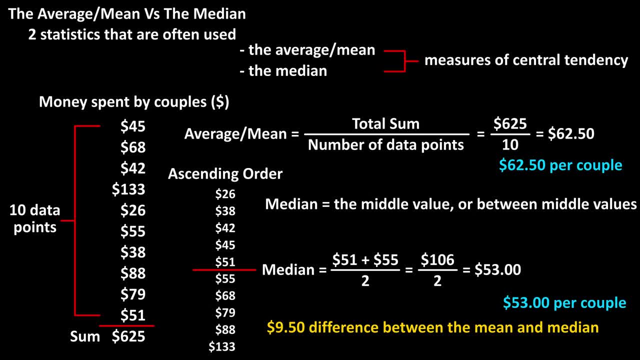 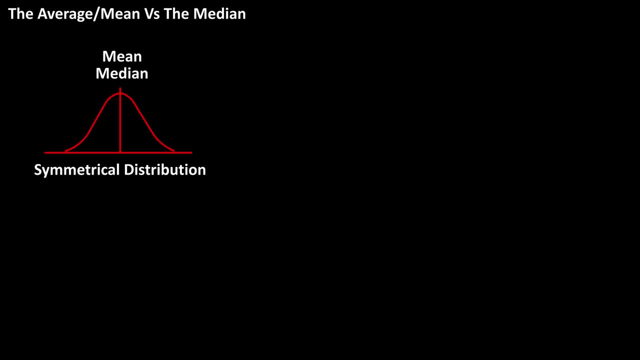 dollars, a nine dollar and 50 cents difference. Both of these tools- the average and the median- can be influenced by the skew of the data. For instance, a symmetrical distribution, as you see in this graph, has some high and some low values and some values in between. 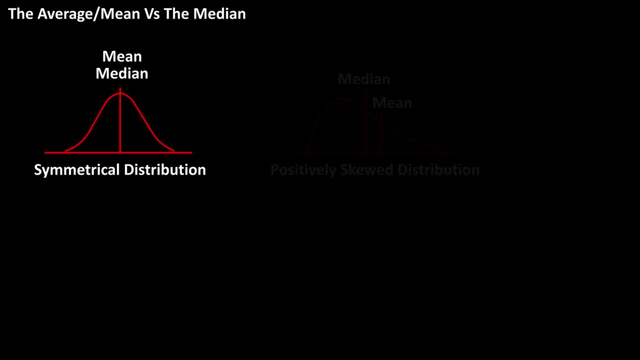 So the mean and the median will lie near the middle. In a positively skewed distribution, the higher values in the data set will pull the mean upwards and the median will be less than the mean more towards the center of the graph. And in a negatively skewed distribution, 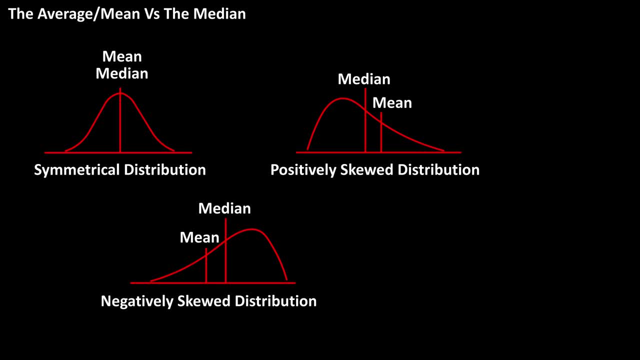 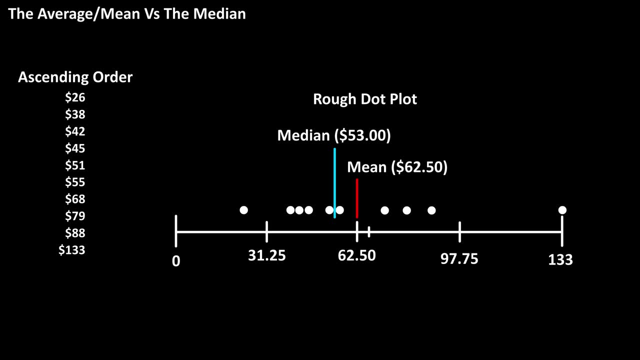 the lower values will pull the mean downwards. the median will again be near the center of the graph, higher than the mean. Here is a very rough dot plot for our example data set of money spent by couples And you can see this: 133 dollar data. 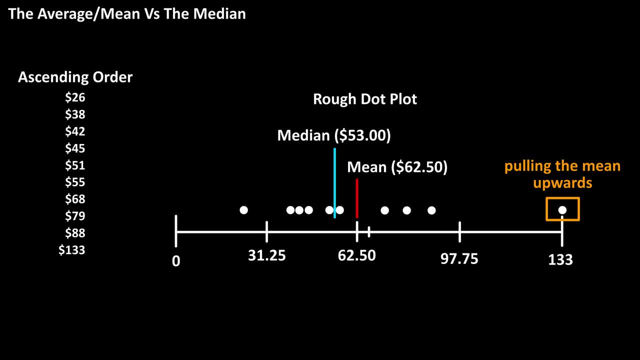 point is really far away from the other data points, So this is pulling the average upwards but it really doesn't have an effect on the median. The mean, or average, is the most used measure of central tendency because it uses all of the values in a data set. 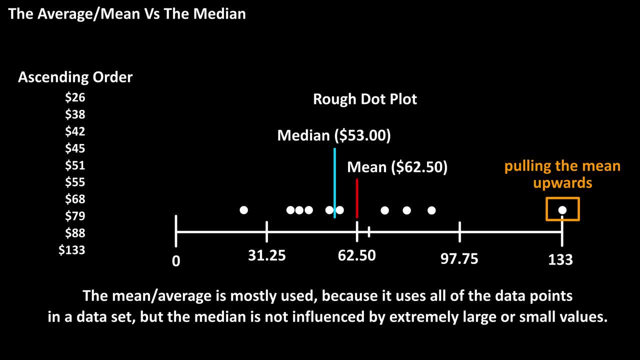 but for data from a skewed data set, the median can be more beneficial because it isn't influenced by extremely large or small values. so the median is less sensitive to outliers, And in statistics it's always a good idea to look at the mean or average.